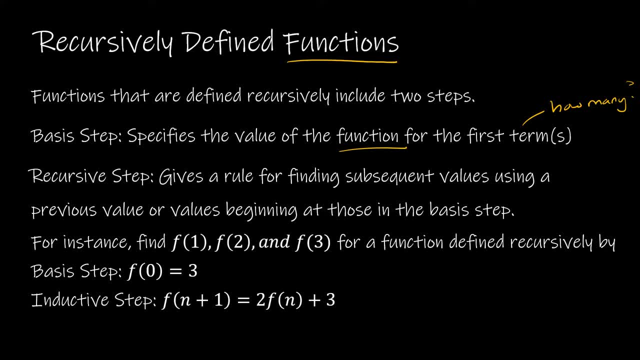 for instance, asks you to take two values, then you would have to have two values in your basis step. And again, for instance, if we have this recursive definition. this recursive definition says the basis step is f of 0 is equal to 3.. Now, before we find f1, f2,. 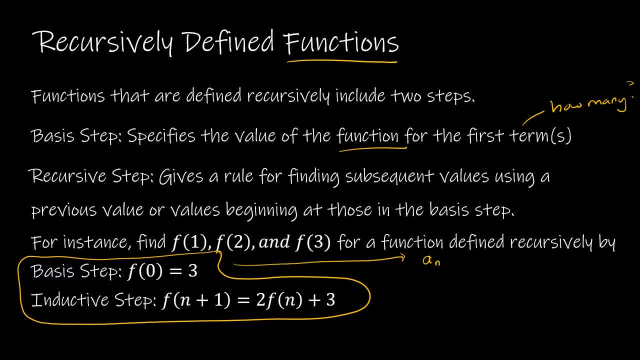 f3,. I want you to notice how similar this is to where we said when we talked originally about sequences: So we took two states in the basis step and we took two classes in the basis step and said a of 0 is 3, and then a of n plus 1 is equal to 2a sub n plus 3.. This is exactly the same thing. 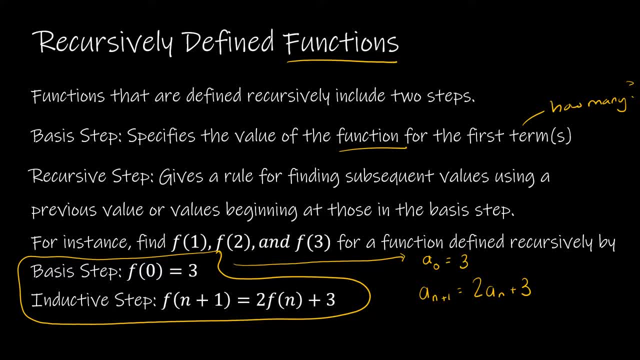 except we're talking about functions instead. but it's really, the process is the same. So for using the inductive step. So F1 says okay, if I have to find F of 0 plus 1, then I'm going to take. 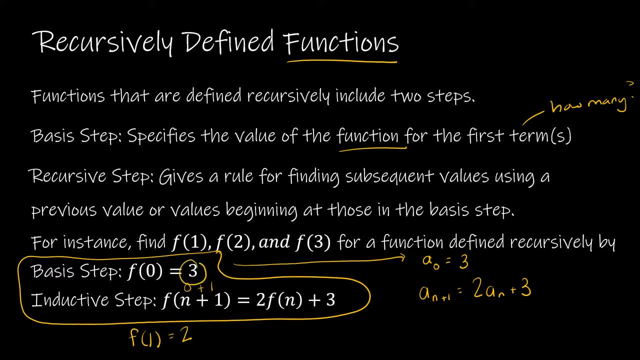 2 times F of 0.. Well, we know F of 0 is 3, and that's why we needed the basis step and then plus 3.. So that's 6 plus 3 or 9.. Now to find F2, that's going to say 2 times F1.. Well, 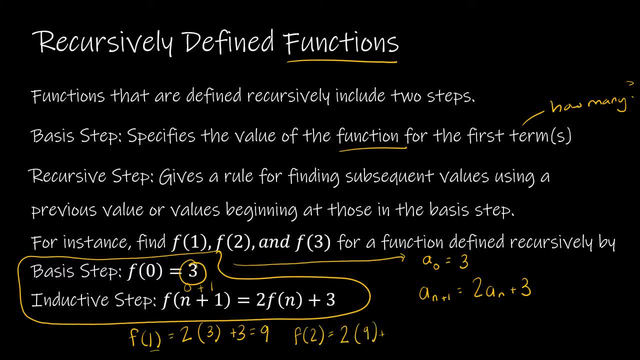 F1 we just determined was 9, and then plus 3.. So that's 18 plus 3 or 21.. And then F3 says to take 2 times F2, which was 21 that we just found, and then plus 3,, which is 45.. 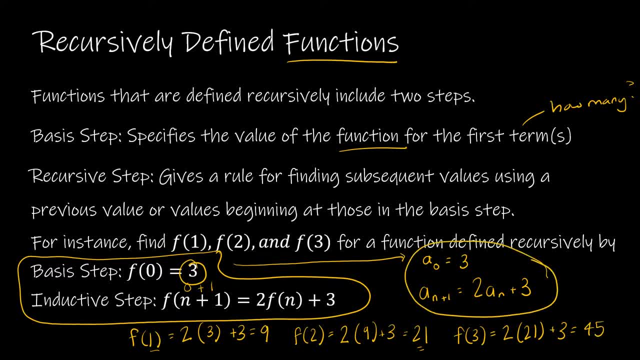 So again the same process that we went through here with our sequences and series, and then plus 3, which is 45. So again the same process that we went through here, and now it's just using functions instead For this first practice, instead of finding 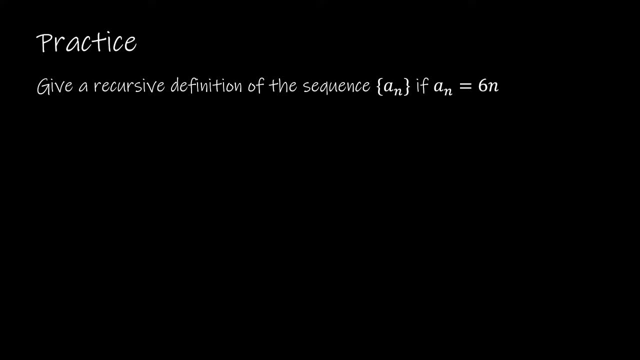 the first few terms of a sequence where it's already been defined for us. they're actually asking us to find the recursive definition of the sequence. So notice, they're giving us the fact that the sequence A sub n is found by taking 6 times n for each value of n. 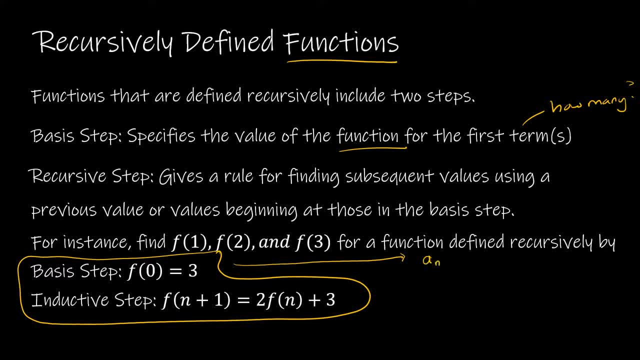 f3,. I want you to notice how similar this is to where we said when we talked originally about sequences: So we said: a of 0 is 3, and then a of n plus 1 is equal to 2, a sub n plus 3.. This is exactly the. 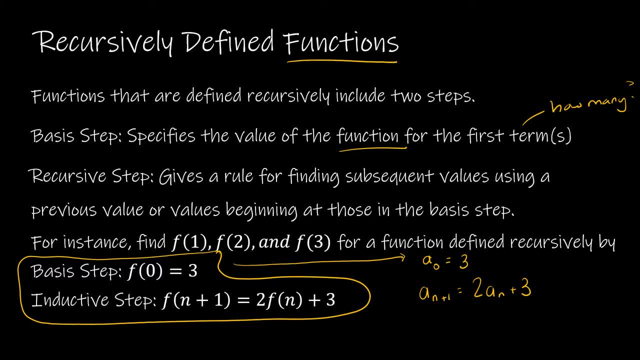 same thing, except we're talking about functions instead. but it's really. the process is the same. So, for instance, this one asks us to find f1 using the inductive step. So f1 says, okay, if I have to find f of 0, then I have to find f of 0.. So f1 says, okay, if I have to find f of 0,. 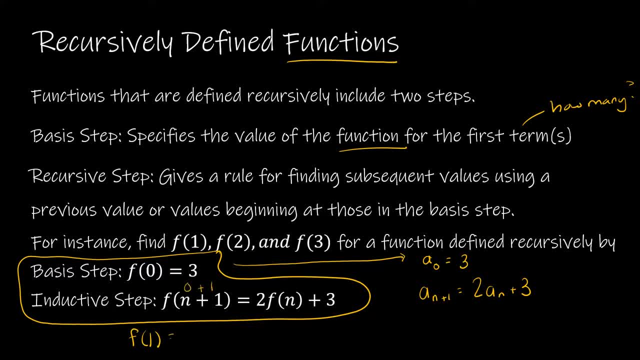 plus 1, then I'm going to take 2 times f of 0.. Well, we know f of 0 is 3, and that's why we needed the basis step and then plus 3.. So that's 6 plus 3, or 9.. Now to find f2, that's going to say 2. 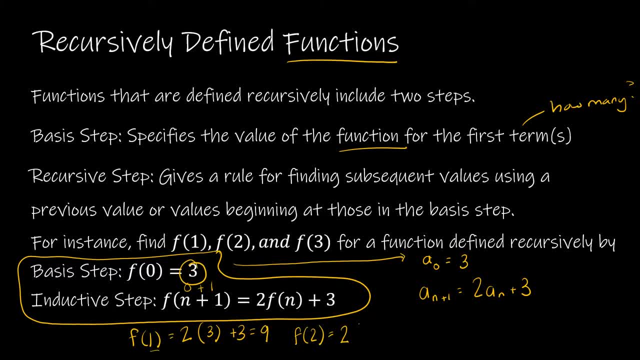 times f1.. Well, f1, we just determined was 9, and then plus 3.. So that's 18 plus 3, or 21.. And then f3, says to take 2 times f2, which was 21,, that we just found, and then plus 3,, which is 45. 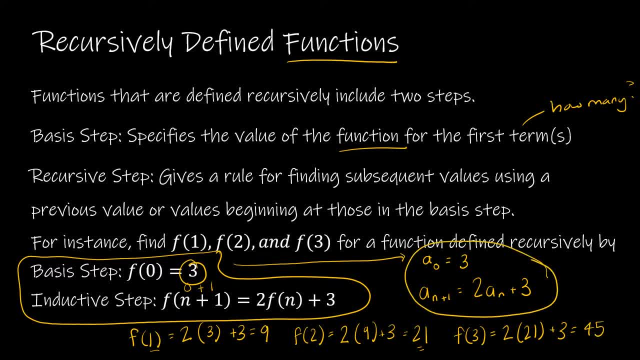 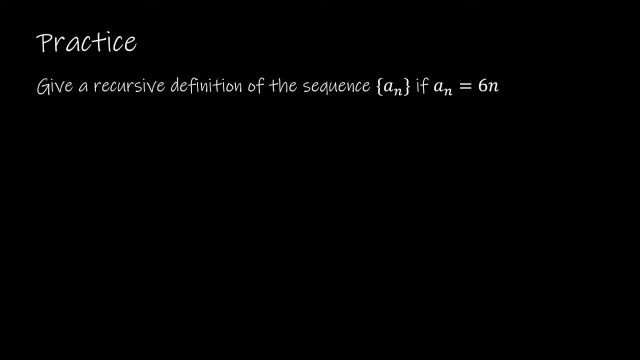 So again the same process that we went through here with our sequences and series, and now it's just using functions instead. So for this first practice, instead of finding the first few terms of a sequence where it's just using functions, instead we're going to find the first few terms of a sequence. 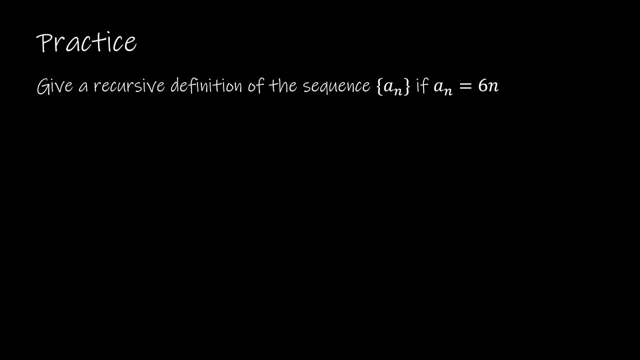 it's already been defined for us. They're actually asking us to find the recursive definition of the sequence. So notice, they're giving us the fact that the sequence, a sub n, is found by taking 6 times n for each value of n. So when they ask us for the recursive definition, remember we're 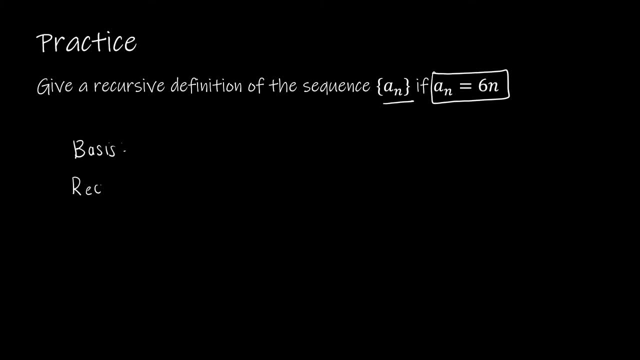 going to have the basis step and the recursive step, And so the basis step should give 1 or 2, or however many values that we need, And the recursive step defines all subsequent values based on the initial value. So before we can do that, let's just find a few values in our set. 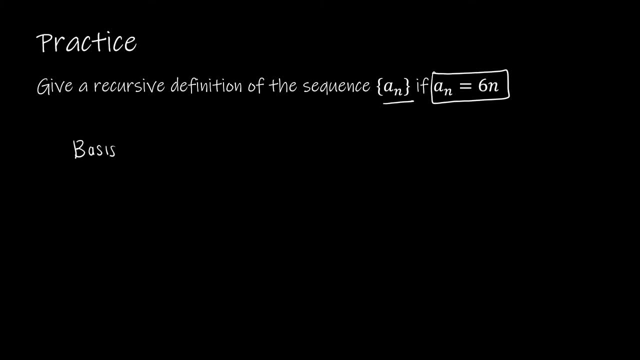 So when they ask us for the recursive definition, remember we're going to have the basis step and then plus 3 times F of 0. So that's going to say 2 times F of 0. And then we're going to have the basis step and the recursive step, And so the basis step should. 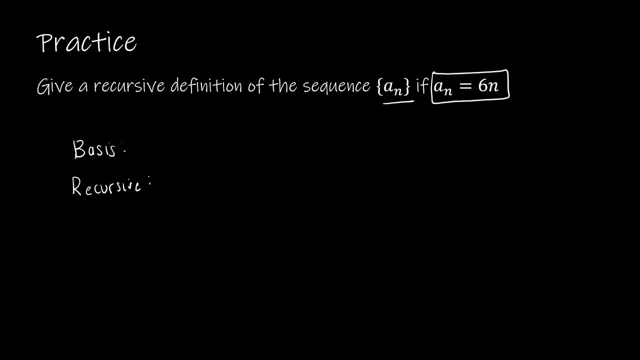 give one or two or however many values that we need, And the recursive step defines all subsequent values based on the initial value. So before we can do that, let's just find a few values in our set. So A0 would be 6 times 0, according to our definition, 6 times 0 is 0.. 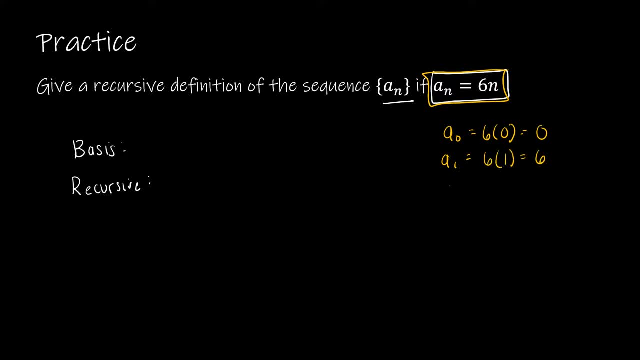 A1 is 6 times 1 or 6.. A2 is 6 times 2,, which is 12.. A3 is 6 times 3,, which is 18.. Now for the basis step. it's pretty straightforward. We know that it's probably. 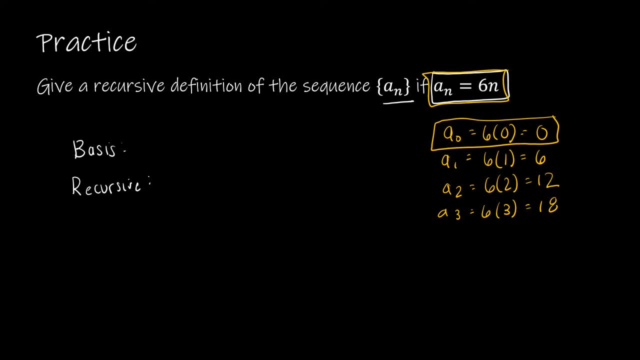 just going to be that our first value is 0. But what you have to be careful of is you should do the recursive step first. So if you're going to do the recursive step first, you should do the recursive step first, because that will tell you how many values you need for your basis. 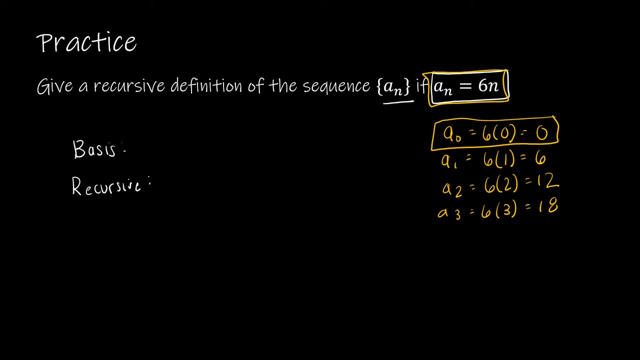 So what we need to do is say: if I'm basing it completely on the previous value, how do I get from 0 to 6?? Again, if I'm basing it on the previous value, how do I get from 6 to 12?? Well, 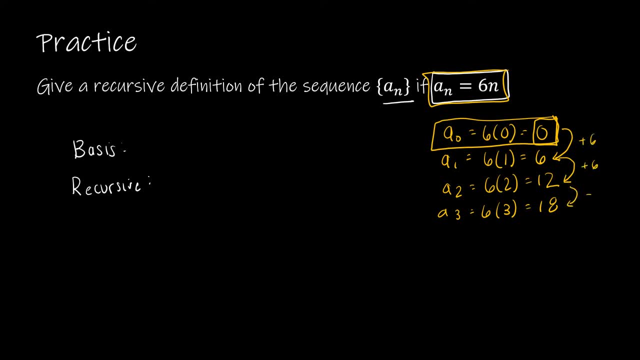 here I've added 6.. Here I've added 6.. Here I've added 6.. So it appears that all I have to do to find F of n plus 1, is to take the value of f of n and add 6 to it. Now, if you'll notice, I've only used one value. 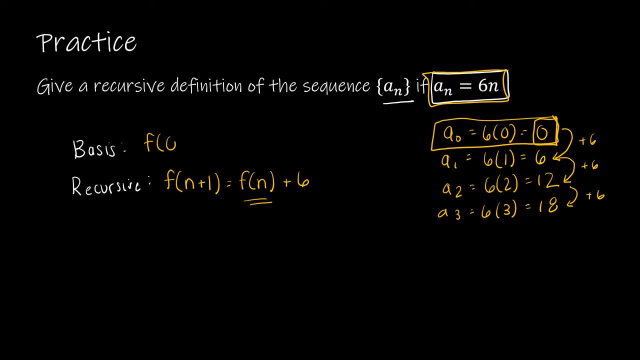 So, because I've only used one value, I'm going to define f of 0 to be 0. And again, you can always go back and test it and make sure you did it right. So, based on this, f of 1 would be 0 plus 6.. 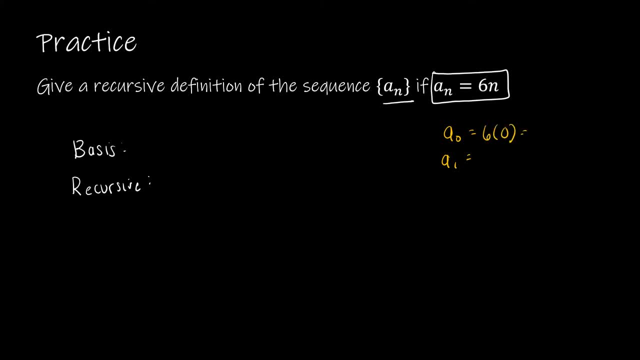 So a0 would be 6 times 0, according to our definition. 6 times 0 is 0.. A1 is 6 times 1, or 6.. A2 is 6 times 2,, which is 12.. 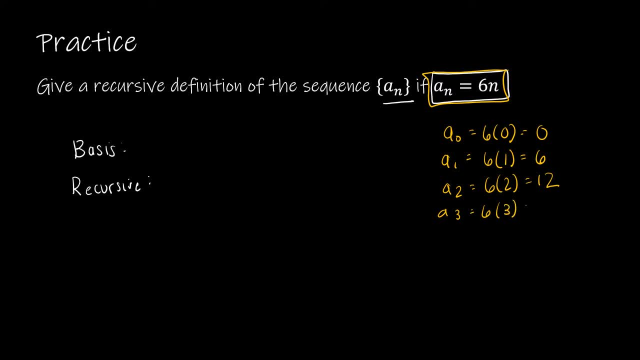 A3 is 6 times 3,, which is 18.. Now for the basis step. it's pretty straightforward. We know that it's probably just going to be that our first value is 0. But what you have to be careful of is you should do the recursive step first, because that will tell you how many values. 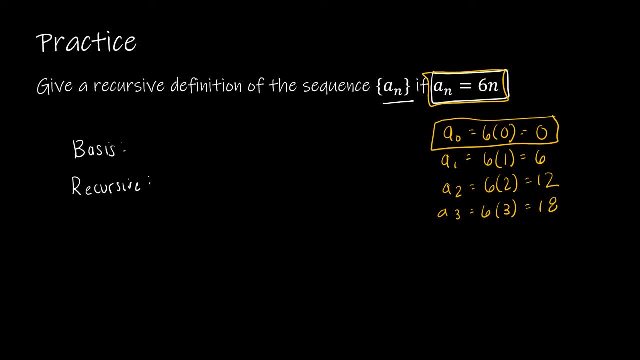 you need for your basis. So what we need to do is say if I'm basing it completely, I'm going to do the recursive step first, because that will tell you how many values you need for your basis. So what we need to do is say if I'm basing it completely on the previous value, how do I get? 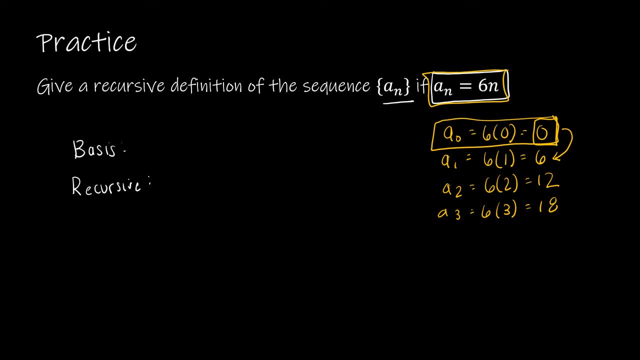 from 0 to 6?? Again, if I'm basing it on the previous value, how do I get from 6 to 12?? Well, here I've added 6.. Here I've added 6.. Here I've added 6.. So it appears that all I have to do 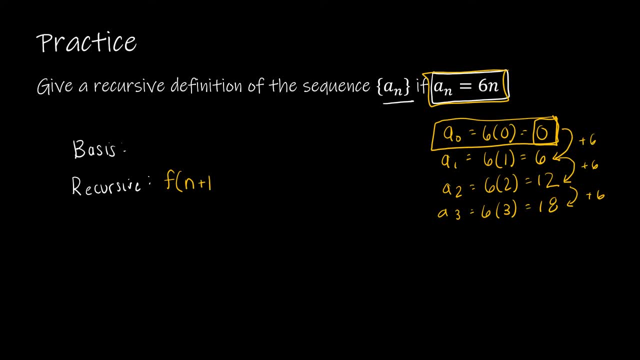 to find f of n plus 1 is to take the value of f of n and add 6 to it. Now, if you'll notice, I've only used one value. So because I've only used one value, I'm going to define f of 0 to be. 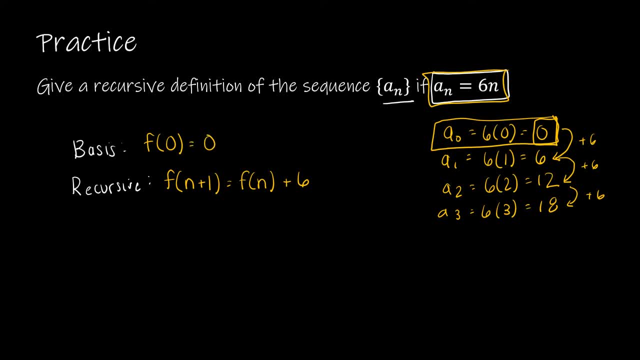 0. And again you can always go back and test it and make sure you did it right. So, based on this, f of 1 would be 0 plus 6. And again, f of 2 would be 6 plus 6. And we can see that we are getting. 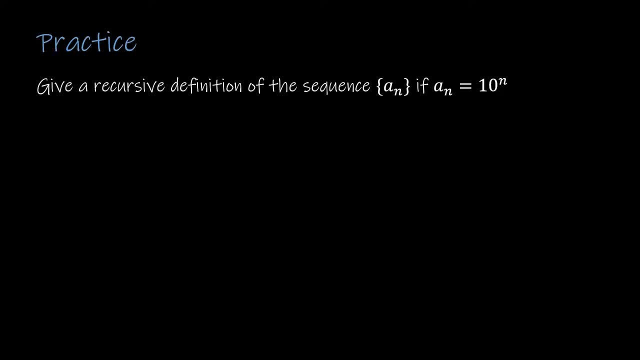 the correct results. Here's a question for you to try. So, if you would press pause, Try this question. then press play to see how you did So. again, we're looking for the two parts, the basis step and the recursive step- And, just like before, we should spend a little bit of time. 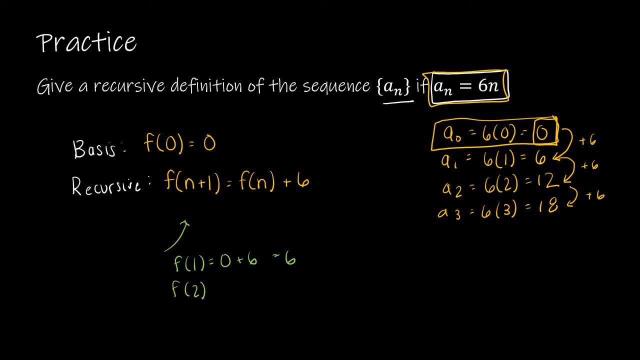 And again, f of 2 would be 6 plus 6.. And we can see that we are getting the correct results. Here's a question for you to try. So if you would press pause, try this question, then press play to see how you did. So again, we're looking for the two parts. 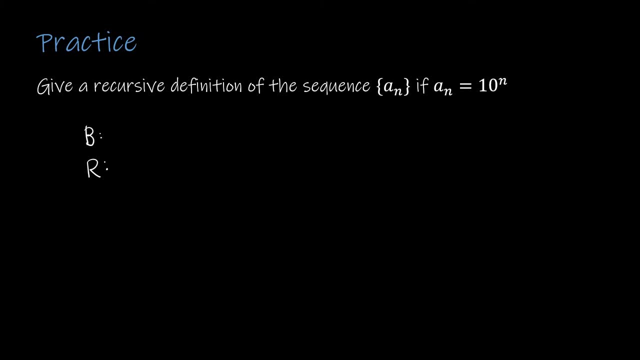 the basis step and the recursive step And, just like before, we should spend a little bit of time finding the correct answer. So if you would press pause, try this question, then press play to see how you did So. again, we're looking for the two parts: the basis step and the recursive step. 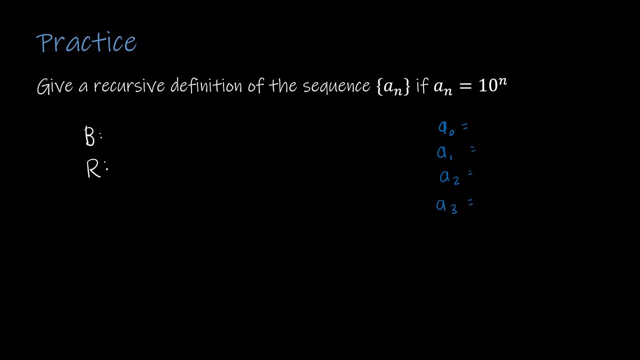 And again we're looking for the two parts: the basis step and the recursive step. And again, we're looking for the two parts: the basis step and the recursive step. So if you would press pause, try this question. then press play to see how you did. 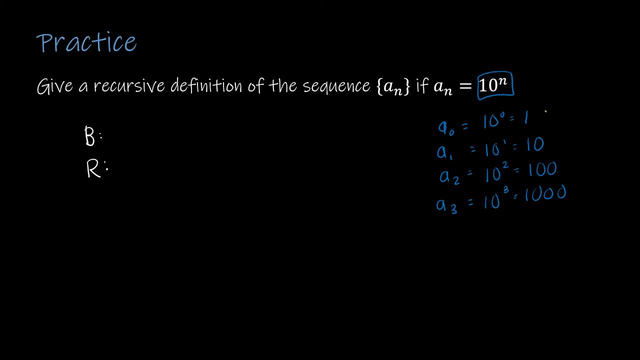 So again, when we're defining things recursively, we're saying: to get from here to here, what did I have to do? Well, it appears that I multiplied by 10.. And to get from here to here, I multiplied by 10.. 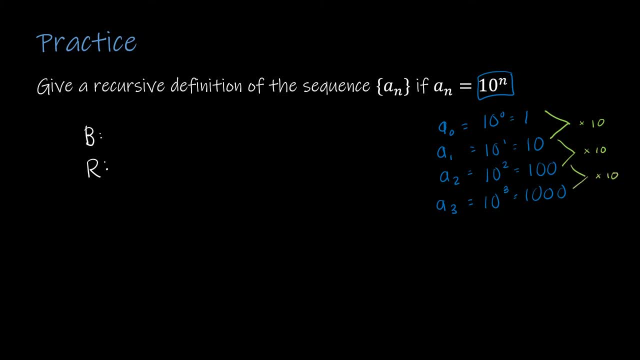 And from here to here I multiplied by 10.. So my basis step is just going to be one value because, as I can see, all I have to do is take one value and multiply it by 10.. So my recursive step f of n plus 1, says: take whatever you had in the step before and multiply it by 10.. 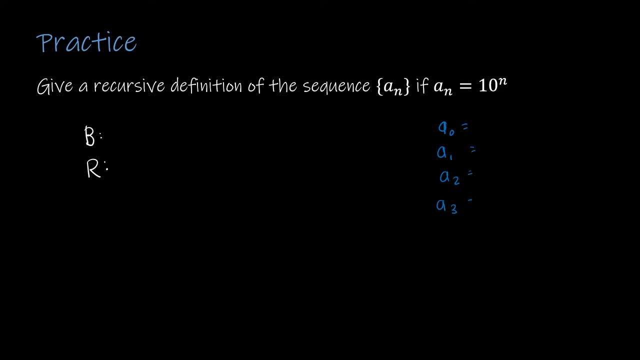 finding the first few values so that we can then come up with some sort of pattern. So we're looking at 10.. to the power of n. So a0 is 10 to the 0, which is 1.. a1 is 10 to the 1st, which is 10.. a2 is 10. 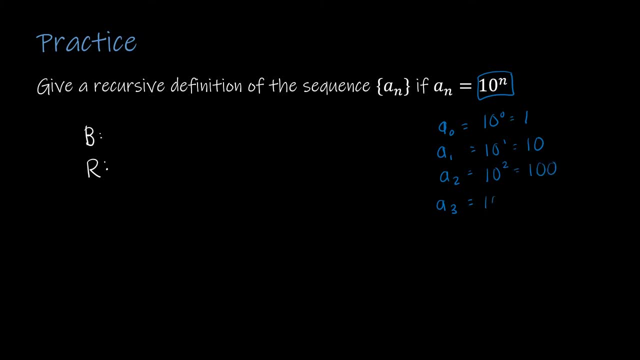 squared, which is 100.. a3 is 10 to the 3rd, which is 1000.. So again, when we're defining things recursively, we're saying, to get from here to here, what did I have to do? Well, it appears. 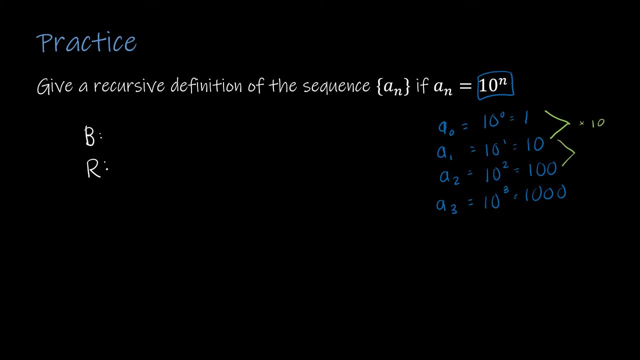 that I multiplied by 10.. And to get from here to here, I multiplied by 10.. And from here to here, I multiplied by 10.. So my basis step is just going to be one value because, as I can see, 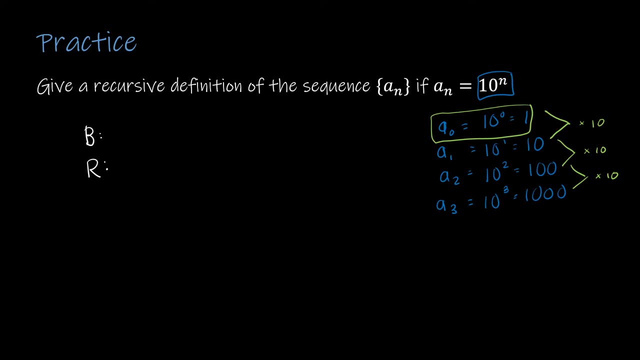 all I have to do is take one value and multiply it by 10.. So my recursive step f of n plus 1, says: take whatever you had in the step before and multiply it by 10.. So I'm going to just put. 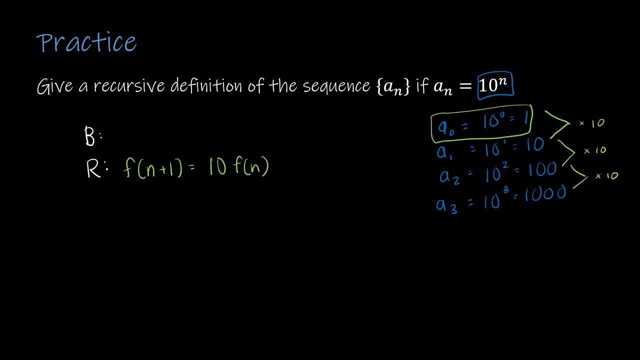 10. f of n. The basis step means I just need one value, because I'm only using one to find the next value. So f of 0 is equal to 1.. And that is your result. Now we're going to take a look. 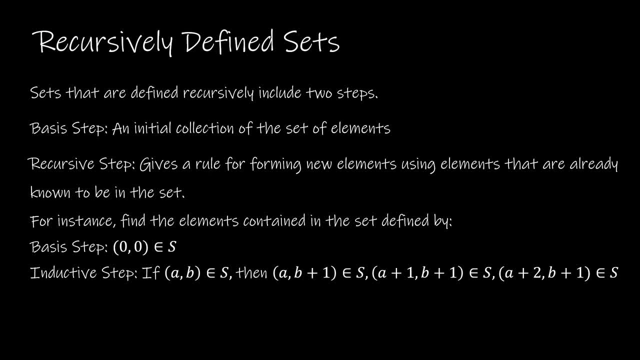 at recursively defined sets And I do just want to point out that the book also covers recursively defined structures and we are not going to cover that in this video. So, again, if I'm looking at recursively defined sets, I'm going to take a look at recursively. 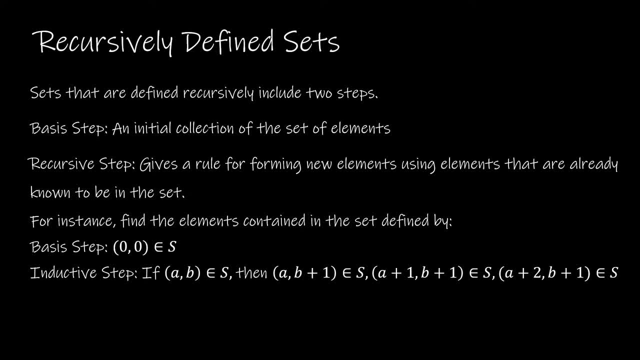 defined structures and we are not going to cover that in this video. So, again, if I'm looking at a set, it's still the same idea. Instead of a function, now, it's a set, The basis step. instead of being a function of a small value, it's an initial collection of the set of elements. 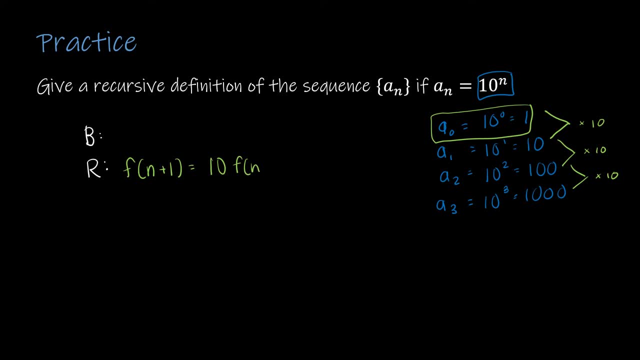 So I'm going to just put 10 f of n. The basis step means I just need one value, because I'm only using one to find the next value. So f of 0 is equal to 1. And that is your result. 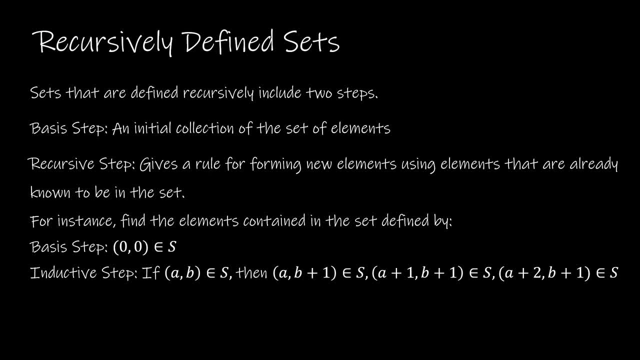 Now we're going to take a look at recursively, And I do just want to point out that the book also covers recursively defined structures and we are not going to cover that in this video. So again, if I'm looking at a set, it's still the same idea. 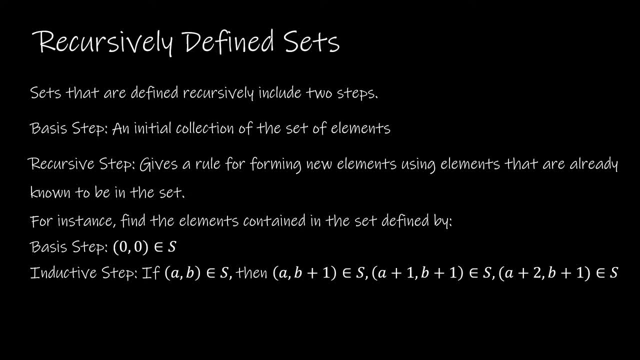 Instead of a function. now it's a set, The basis step, instead of being a function of a small value. it's an initial collection of the set of elements, And the recursive step just says here's how to find new elements in the set based on ones that are already in the set. 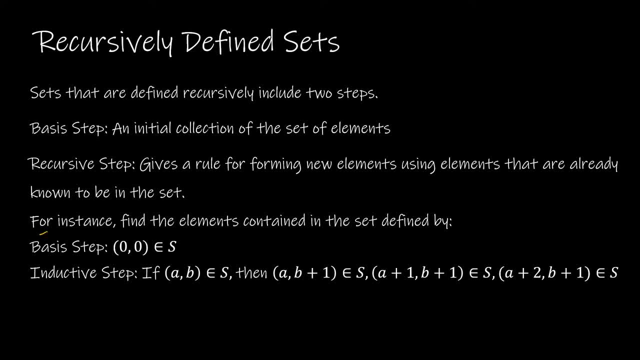 So we're going to take a look at this example And this example is going to be very important because we're going to continue looking at this example in the next video. So you might feel like I'm sort of beating a dead horse as I go through this example and I apologize for that. 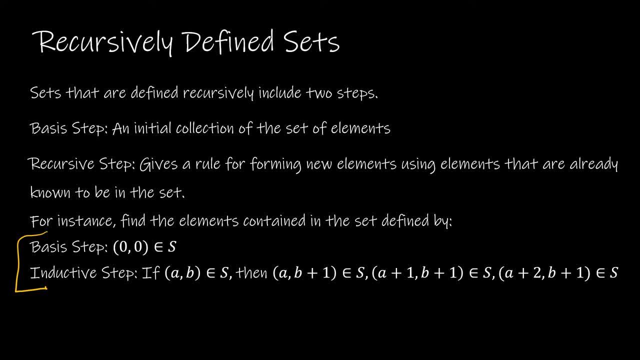 But it's so that we can talk about it again in the next video. So this asks us to find the elements contained in the set defined by the basis step, which is that 0, 0 is in the set, So basis Tells me 0, 0.. 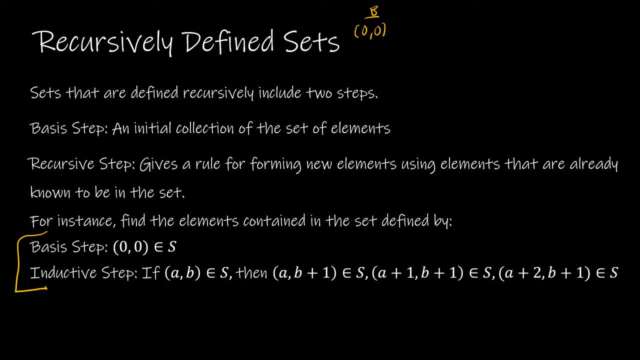 And then the inductive step is: if a comma b is in the set, then a comma b plus 1, a plus 1 comma b plus 1, and a 2 comma b plus 1 is in the set. So let's find what happens when we do our first run through using 0, 0. 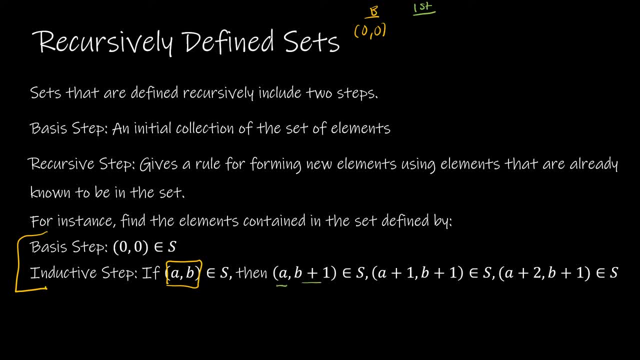 So notice: a is going to stay the same. I'm going to add 1 to b, A is going to add 1. And I'm going to add 1 to b, And a is going to add 2.. And I'm going to add 1 to b. 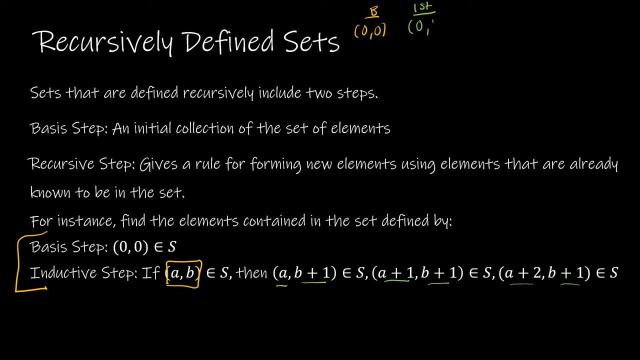 So this is going to give me: a is the same and add to b. A is plus 1, add to b. A is plus 2, add to b. So that's what happens my first time through. Then I'm going to take those values. 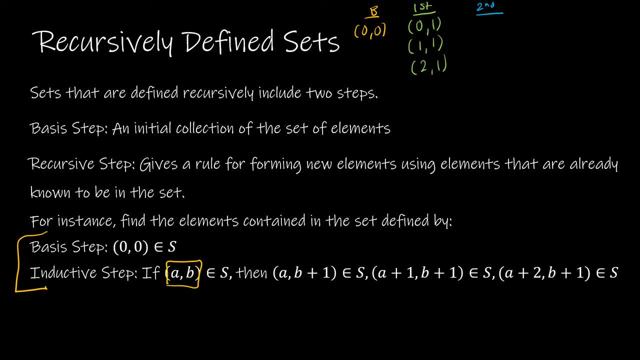 And I'm going to do the same thing, And obviously we're not going to find all of the elements in the set, because this set is going to be the same. The one we're going to need to do is'th, and the second set is going to be the same: the. 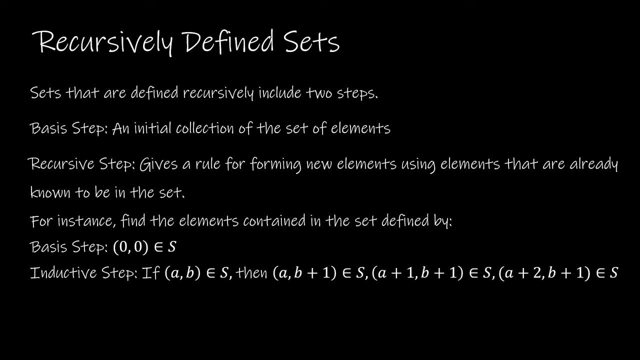 And the recursive step just says: here's how to find new elements in the set based on ones that are already in the set. So we're going to take a look at this example And this example is going to be very important because we're going to continue looking at this example in the next. 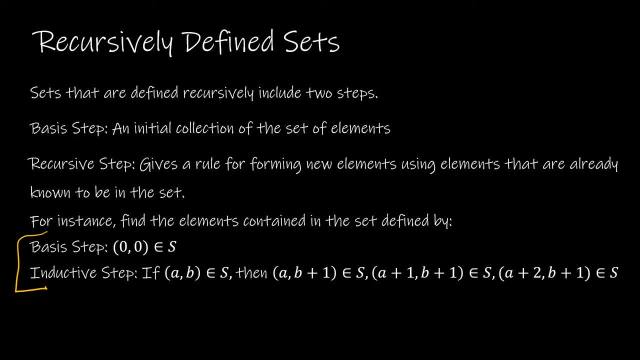 video. So you might feel like I'm going to be doing a lot of work on this, but I'm not. I'm sort of beating a dead horse as I go through this example and I apologize for that, but it's so that we can talk about it again in the next video. So this asks us to find the elements. 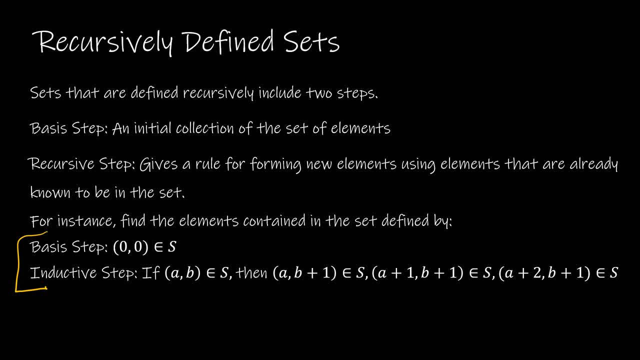 contained in the set defined by the basis step, which is that 0, 0 is in the set. So basis tells me 0, 0.. And then the inductive step is: if a comma b is in the set, a comma b plus 1, a plus 1 comma b plus 1, and a 2 comma b plus 1 is in the set. 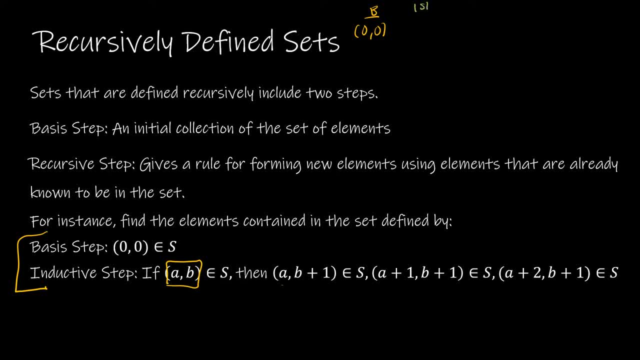 So let's find what happens when we do our first run through using 0, 0.. So notice: a is going to stay the same, I'm going to add 1 to b, a is going to add 1, and I'm going to add 1 to b. 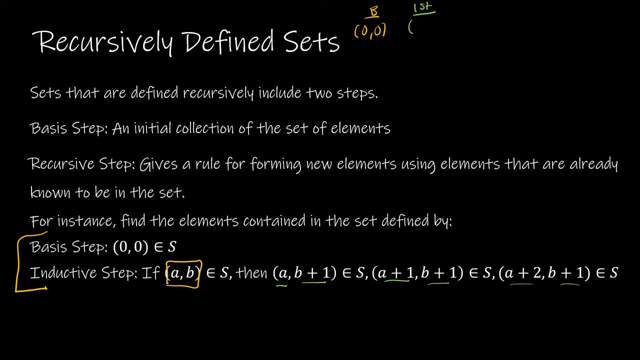 and a is going to add 2, and I'm going to add 1 to b. So this is going to give me: a is the same and add to b. a is plus 1, add to b plus 2, add to B. so that's what happens my first time through. then I'm going to 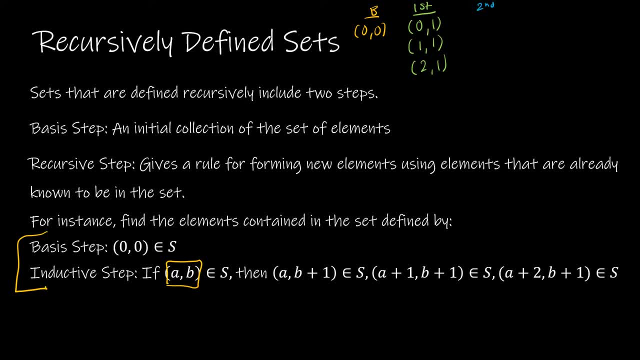 take those values, and I'm going to do the same thing, and obviously we're not going to find all of the elements in the set, because this set is infinite, right, because that we can just keep adding, and adding, and adding. but what we're doing is we're looking for a pattern. how can we sort of define or talk about what's? 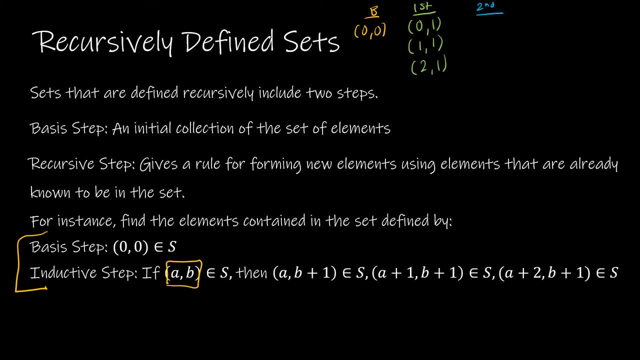 in the set and we, in order to do that, we have to find some of the values that are in the set. so again, a is going to. so I'm going to start with 0, 1. a is going to stay the same and I'm going to add 1 to B. a is going to stay the same, I'm. 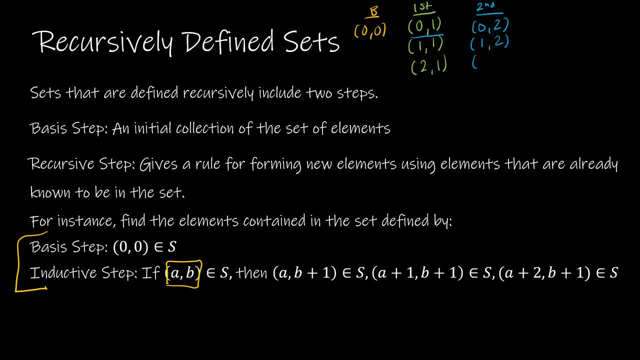 sorry, a is going to add 1 and I'm going to add to B, and a is going to add 2 and I'm going to add to B. now I'm going to do the same thing with 1- 1. so a is going to stay the same and I'm going to add one to B, but that would just give me one, two, so I'm not. 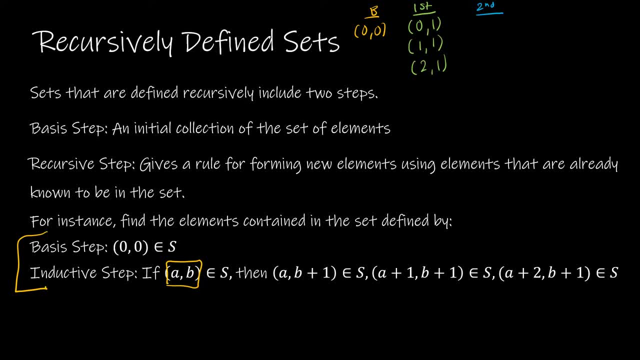 That is 2 plus 1 over 2 minus 2 and give us 2.. And we're going to put all of these values together to get something like that. We want to masterlü heyforum. That will make things True. 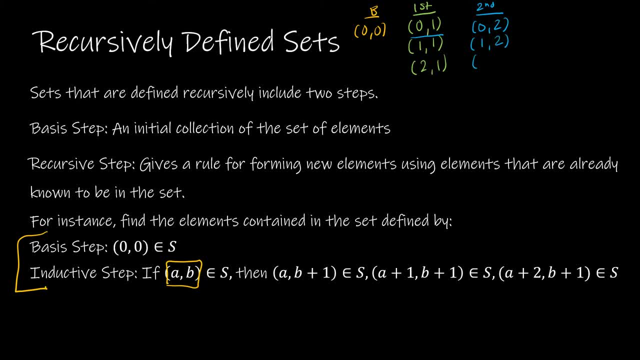 In fact, we're going to make a pattern Right, and A is going to add 2, and I'm going to add to B. Now I'm going to do the same thing with 1, 1.. So A is going to stay the same and I'm going to add 1 to B, but that would just give me 1, 2,. 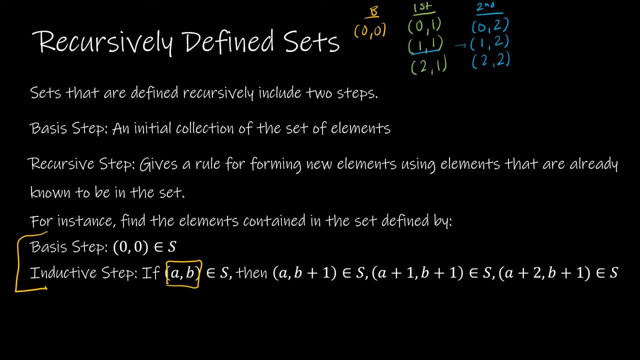 so I'm not going to write it again. And then A is going to stay this, or A is going to add 1, so that's 2, and I'm going to add 1 to B, so that's 2, 2.. Yep, we already have that one, And 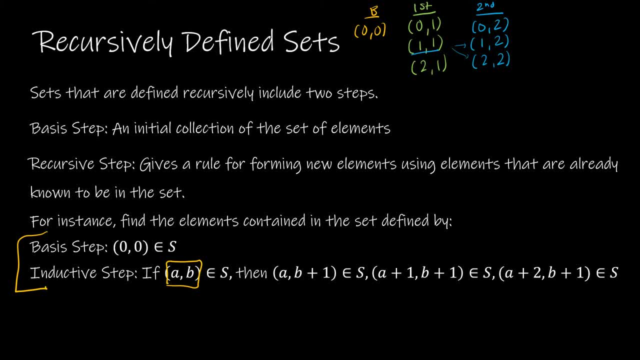 then A is going to add 2,, so that's 3, and then add 1 to B, so that's 3, 2.. And then I'm going to look at 2, 1, and I'm going to do the exact same thing. So for 2, 1,, A is going to stay the same. 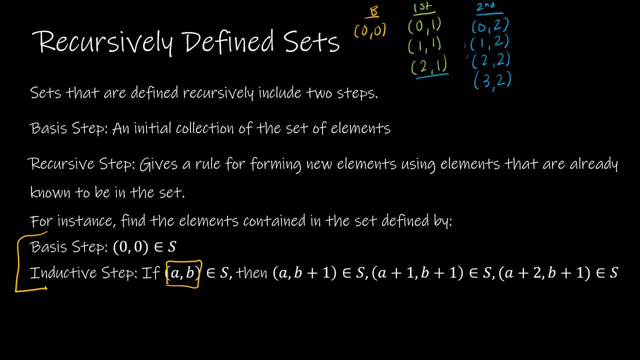 and I'm going to add 1 to B, so that's 2, 2.. We already have it. A is going to increase by 1,, so that's going to be 3, 2.. I already have it, And A is going to increase by 2,, so that's. 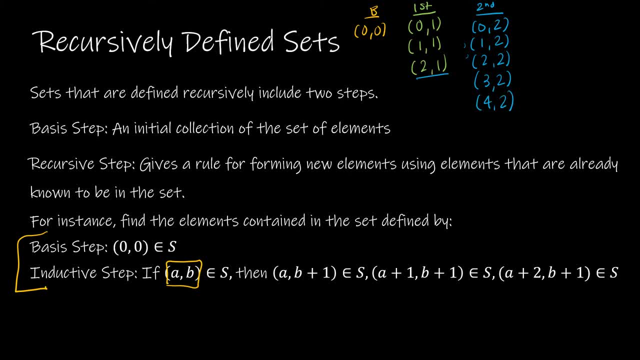 4, 2.. So hopefully you're kind of seeing a pattern. For a last value of 0,, the first value is 0.. For a last value of 1, or a second value, in our ordered pair we have 0,, 1, and 2.. For our second value, 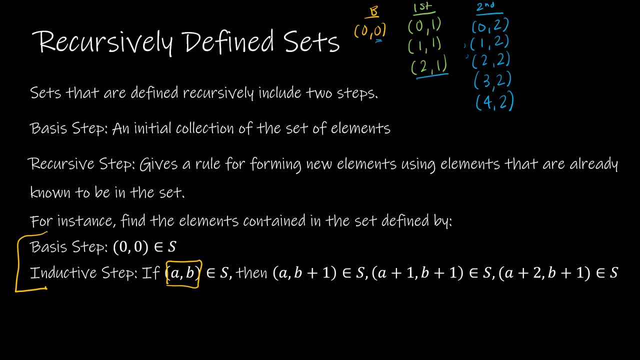 of 2, we have a first value in the ordered pair of 0,, 1,, 2,, 3, and 4.. So what I'm kind of seeing here is that, whatever this second value is, this second value is going to be 0,, 1,, 2,, 3, and 4.. 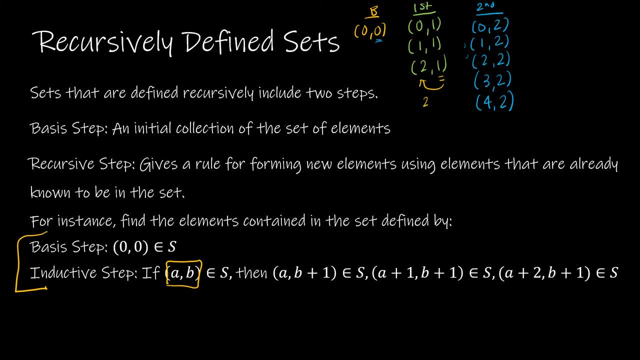 This is going to be 2 times that second value or less. So here, 2 times 2 gives me 4, and notice, it's 4 all the way down. So let's just test that theory. Let's find our third iteration. 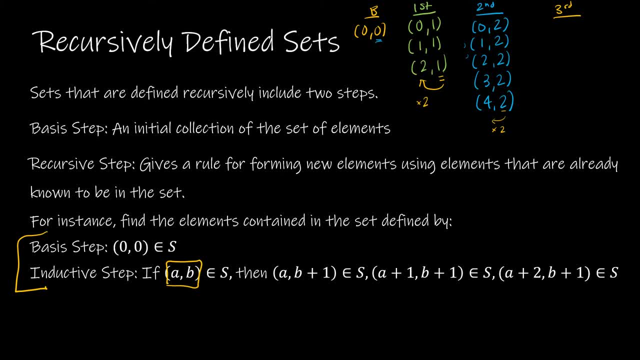 So if we look at our third iteration, A stays the same and we're going to add 1 to B, A adds 1, and we're going to add 1 to B And A adds 2, and we're going to add 1 to B, Then I'm going to do: 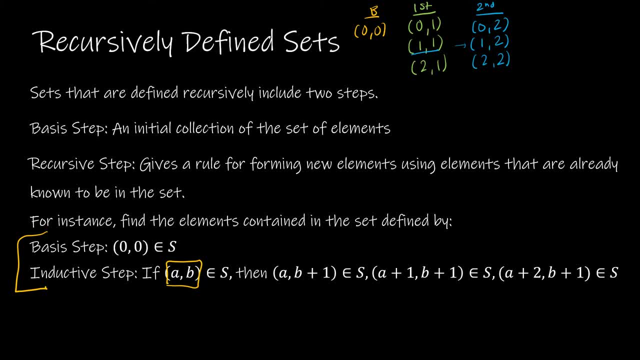 going to write it again. And then A is going to add one, so that's two. and I'm going to add one to B, so that's two, two. Yep, we already have that one. And then A is going to add two, so that's. 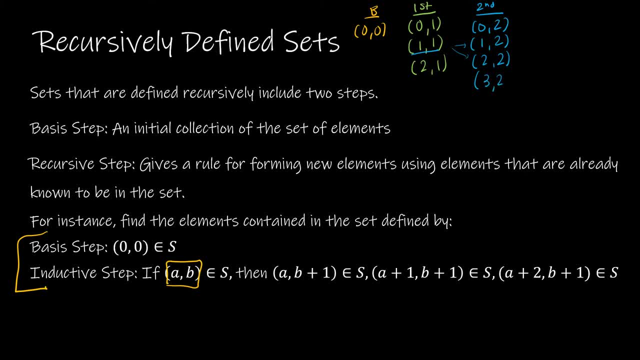 three and then add one to B, so that's three comma two. And then I'm going to look at two one and I'm going to do the exact same thing. So for two, one A is going to stay the same. 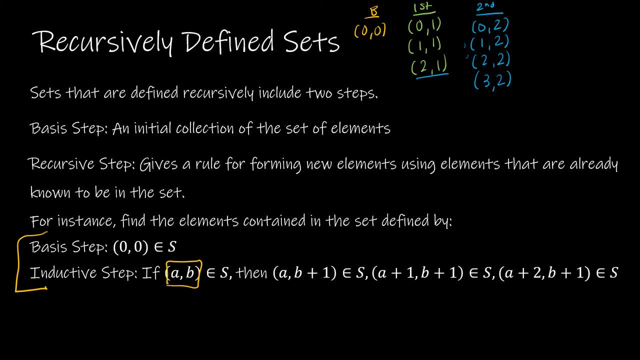 and I'm going to add one to B, so that's two. two- We already have it. A is going to increase by one, so that's going to be three. two- I already have it. And A is going to increase by two, so that's. 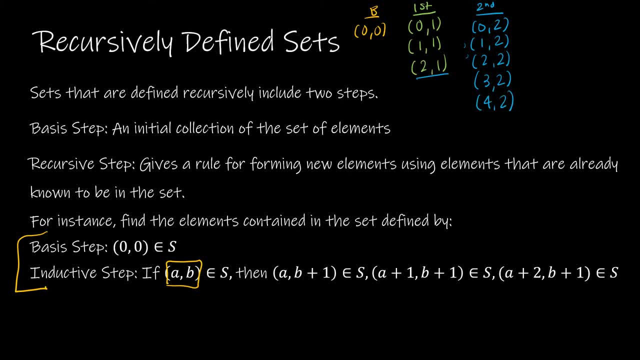 four, two. So hopefully you're kind of seeing a pattern. For a last value of zero, the first value is zero. For a last value of one or a second value, in our ordered pair we have zero one and two For our second value of. 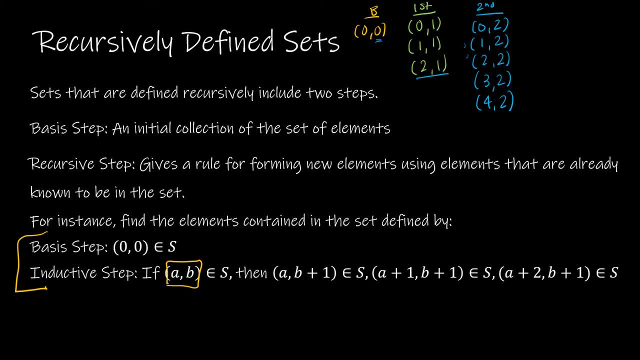 two. we have a first value in the ordered pair of zero: one, two, three and four. So what I'm kind of seeing here is that, whatever this second value is, this is going to be two times that second value or less. So here, two times two. 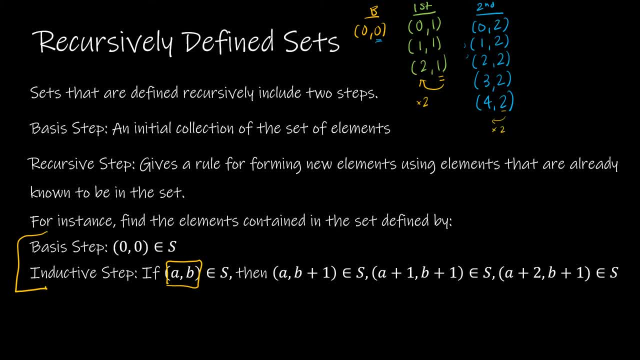 gives me a second value of two. So I'm going to add one to B, and I'm going to add one to B and notice it's four all the way down. So let's just test that theory. Let's find our third. 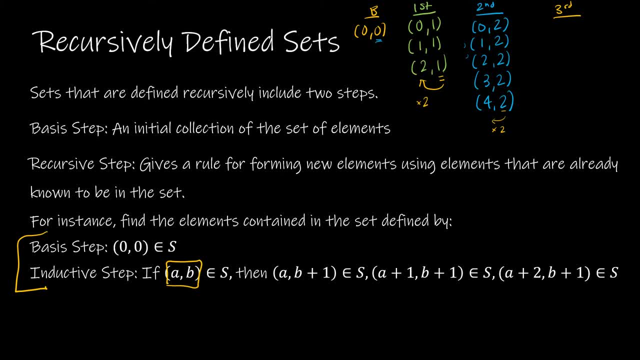 iteration. So if we look at our third iteration, A stays the same and we're going to add one to B, A adds one and we're going to add one to B. Oh, sorry, that's three, And A adds two. 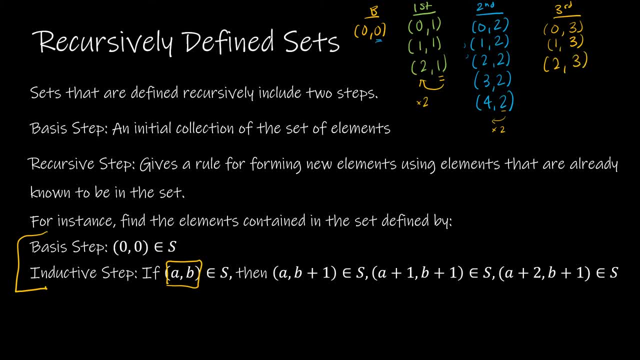 and we're going to add one to B, Then I'm going to do the same for one and two. So A stays the same and we add one, A adds one and we add one. So that's two, three. 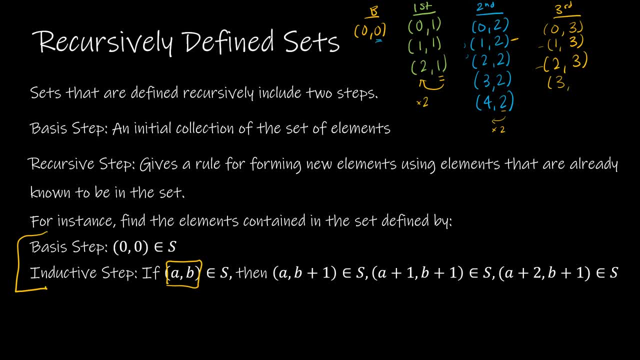 And then A adds two and we add one- Oops, I'm confusing myself. So three, three. Now I'm going to move on to two, two, A stays the same and I add one, So that's two, three. 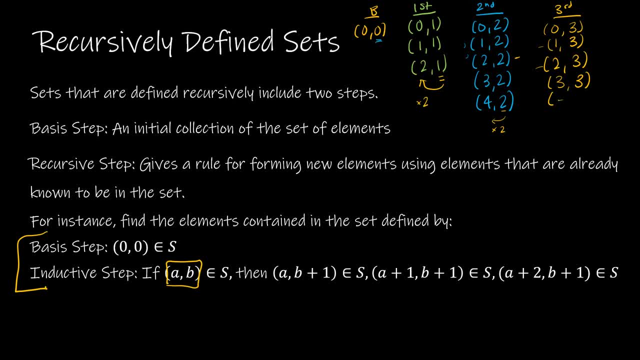 And then three, three, and then four, three, And now I'm moving on to three, two, So that's three, three, four, three and five, three, And then I move on to four, two, and that gives me four, three, five three and six, three. 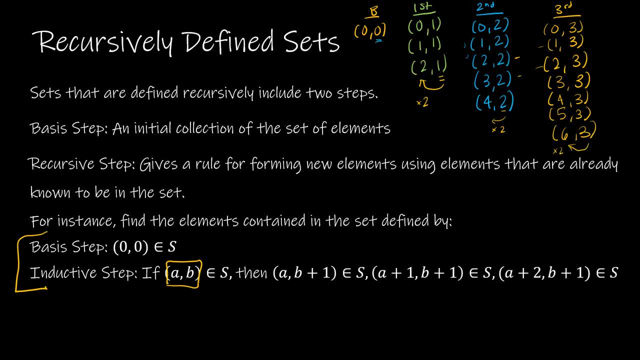 And so again, do I notice that same pattern? I do, So we'll talk about this again in our next video on structural induction. But what seems to be happening is, in the case of A comma, B, that's in the set, it seems to be that A is less than or equal to two B. 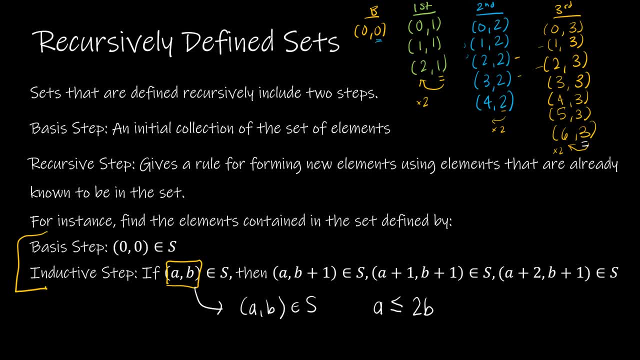 So again, if I take the second value and I multiply it by two, A is going to be less than or equal to that, And that certainly holds true here. Six is equal to that and all of the values less than that are obviously less than Same thing here. 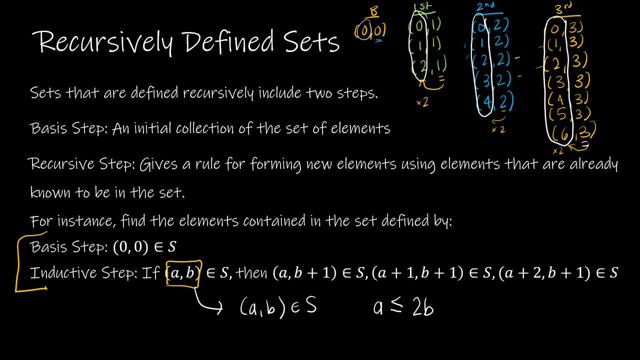 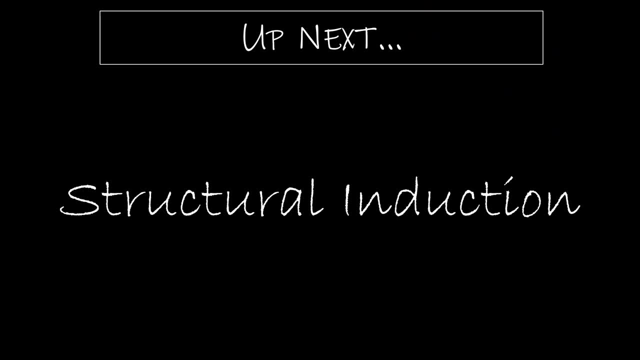 Same thing here, Same thing here Up. next we're going to look at structural induction, which is another type of mathematical induction using recursive definitions. 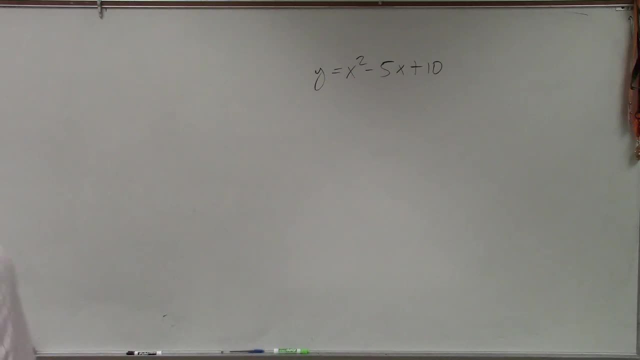 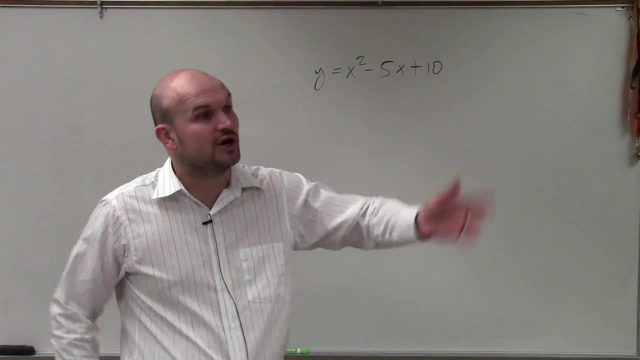 So the first thing, ladies and gentlemen, we want to do is: y equals x squared minus 5x plus 10.. Now we're going to be able to solve this. Now what we learned in this class so far, which will have our test, which will be next class period, regarding solving factoring by GCF. 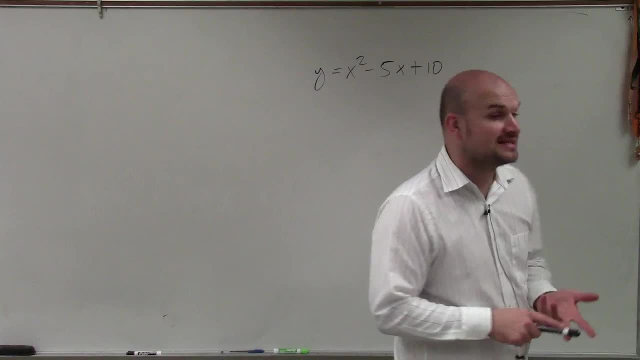 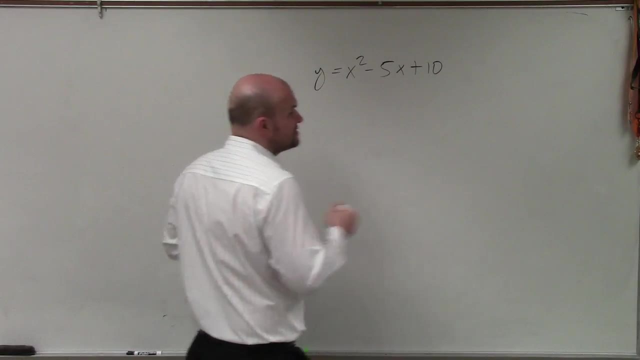 factoring a trinomial when a equals 1,, factoring a trinomial when a does not equal 1, and as well as including the quadratic formula, which we're about to go over today. Now, if I was going to typically go ahead and solve this by factoring, 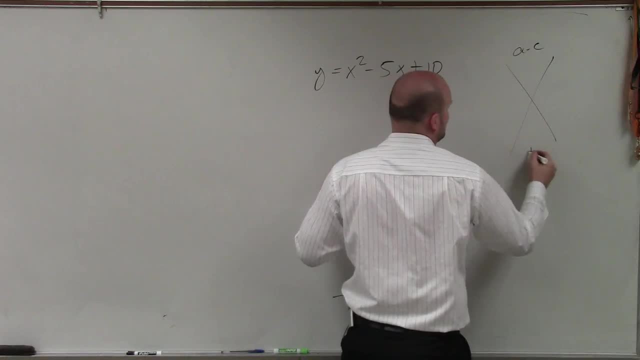 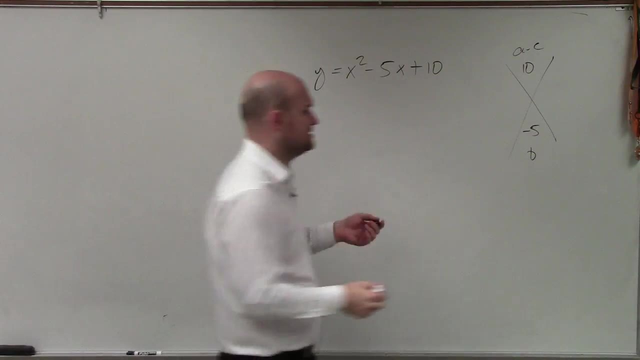 you know, I'd create your nice little diamond here and I'd say my a times c and my b, and if you guys remember, we'd multiply. What two numbers? multiply to give you 10, but then add to give you negative 5? Well, when we start listing our factors of 10,, 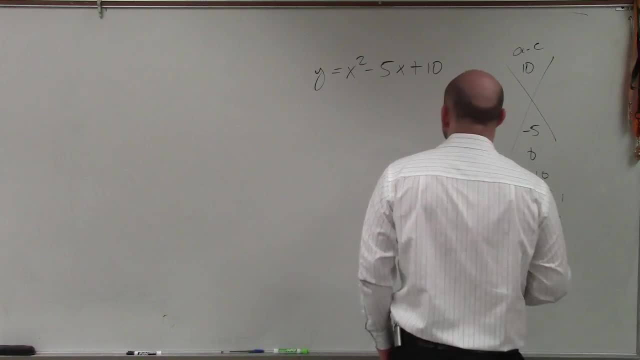 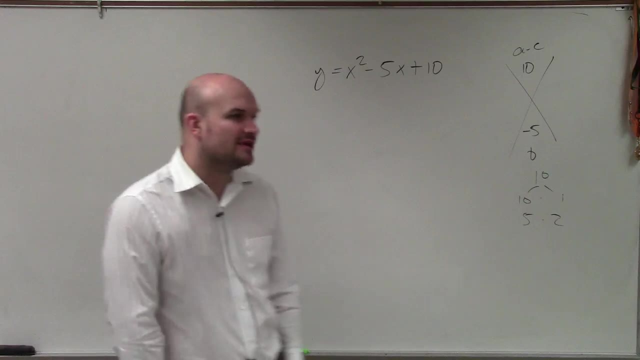 I do 10 times 1,, 5 times 2, and it kind of comes up to me crap. there is not any numbers in the real number system that multiply to give you 10, but add to give you negative 5..